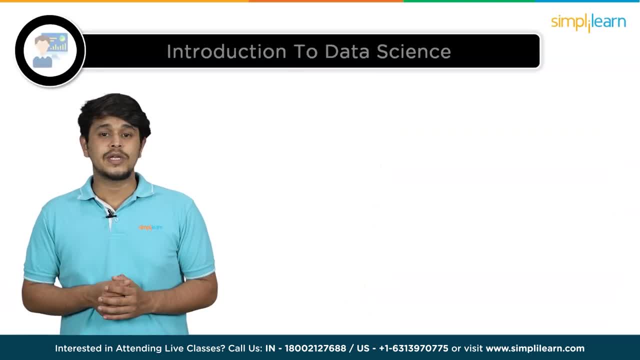 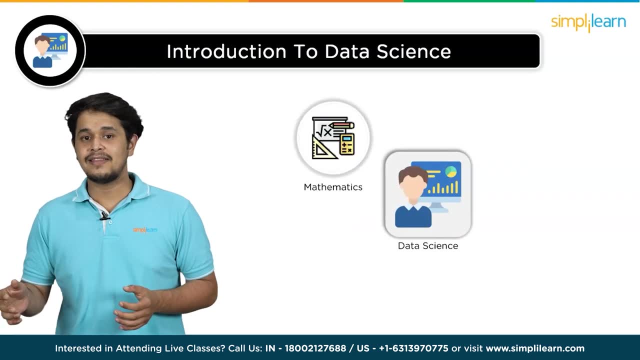 make a career in any of these fields. So let's start with data science. Data science helps businesses understand and utilize data effectively. It uses techniques from math, statistics, AI and engineering to analyze large datasets. By doing this, data scientists can discover insights about 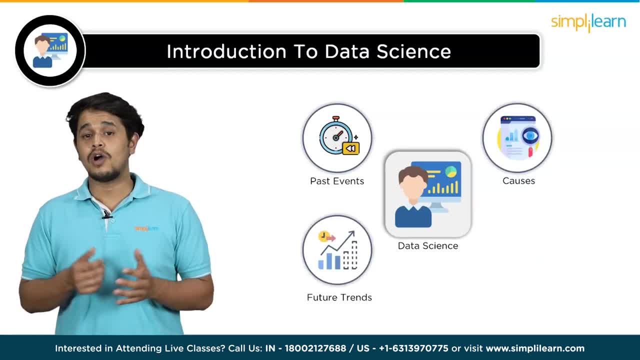 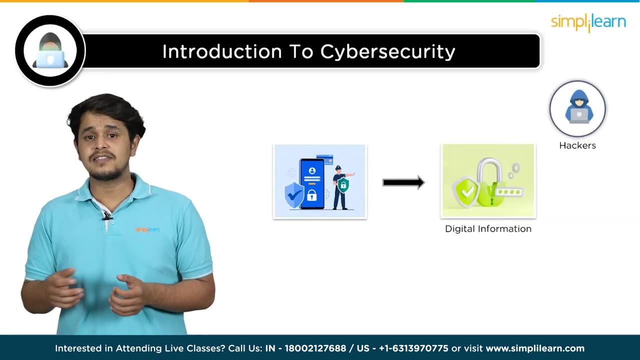 past events, their causes, future trends and how to apply the information. Data science empowers companies to make informed decisions and tackle challenges successfully by leveraging the potential of data. Cybersecurity, on the other hand, safeguards your digital information from hackers and threats. It includes measures like strong password firewalls, antivirus software and 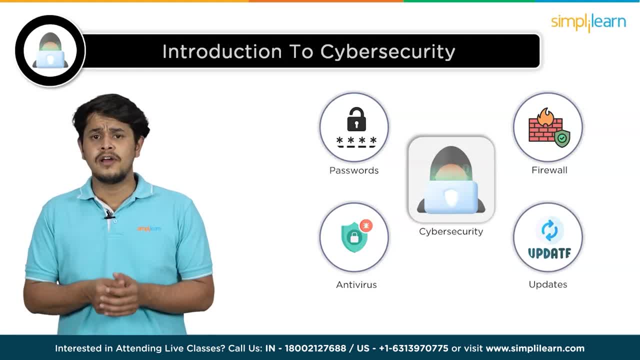 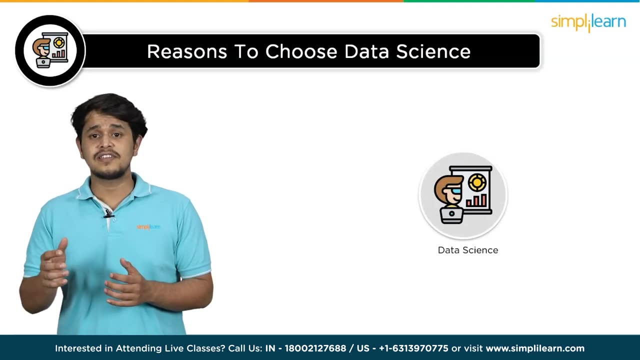 against unauthorized access, viruses and malware. Practicing good cybersecurity ensures a safer online experience and prevents your personal information from being compromised. So let's see the reasons to choose data science as a career. Not just salary, but there are various reasons to consider data science as a career option: High demand: The demand for data scientists is 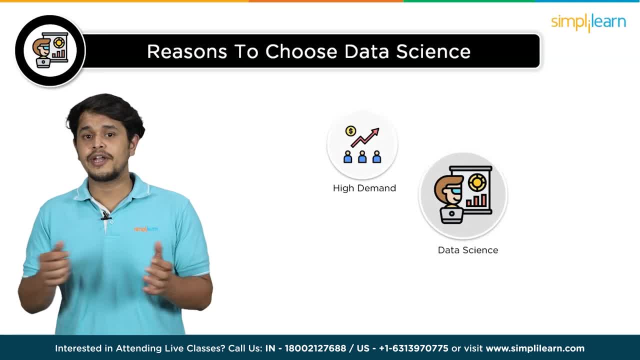 rapidly increasing, with the projected growth of 36% from 2021 to 2031.. According to the Bureau of Labor and Statistics, this makes data science a highly sought-after career choice. Job security Data science is a fast-growing field, As highlighted in LinkedIn's annual Jobs on the Rise report. 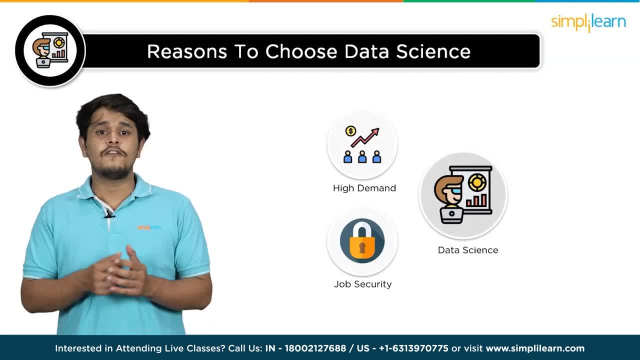 with machine learning engineers, ranking fourth. the field offers strong job security and promising growth opportunities. Diverse job opportunities. Studying data science opens up many job opportunities, including roles such as data scientists, data analysts, data engineers, data architects, business intelligence and data security. Data science is a highly sought-after career choice. 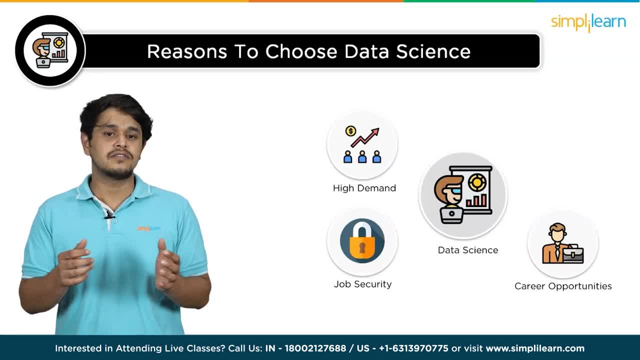 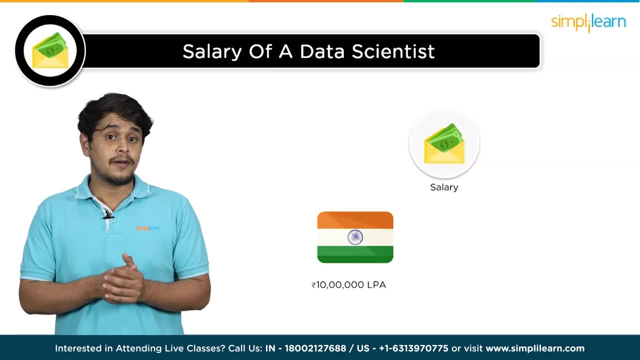 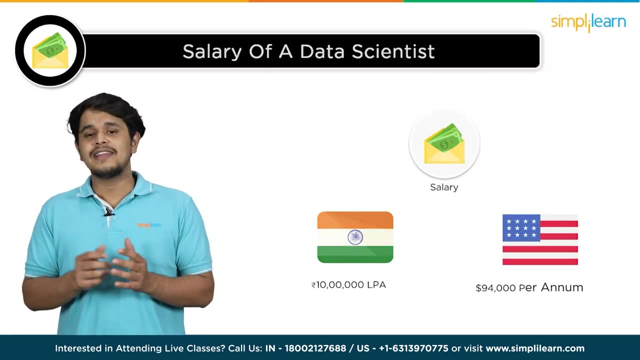 You are a data science analyst, database administrator and machine learning engineer. You have a creative career. The average salary of a data scientist in India goes up to 10 lakh per annum. In contrast, the same data scientist in the United States earns $94,000 per year. with 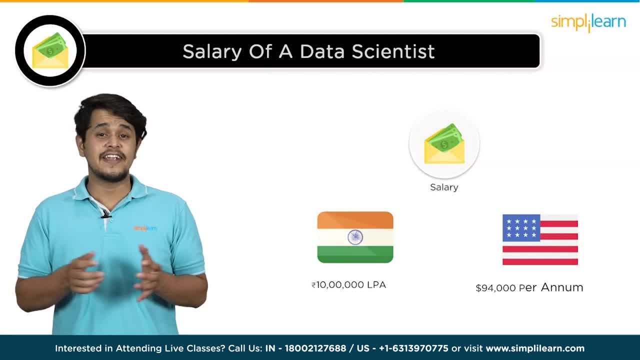 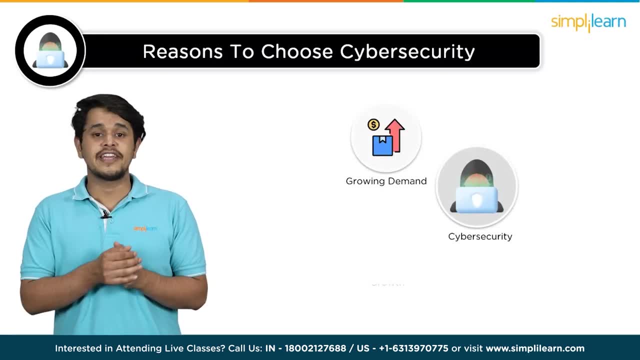 additional cash benefits. So are these reasons enough to consider data science as your career? Or let me just walk you through the reasons to learn cybersecurity: The growing demand for cybersecurity experts. The demand for Cybersecurity specialist is growing rapidly, with an estimated 32% growth from 2018 to. 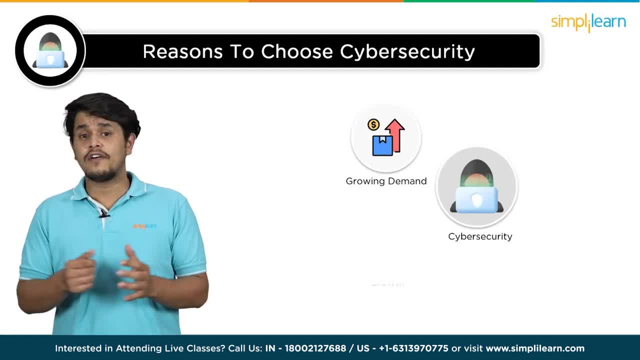 2028.. These reports are according to the Bureau of Labor Statistics. This surge in demand is driven by the continuous expansion of our digital world, with more websites, applications and users sharing sensitive information. online Opportunities for growth and mobility. Fortunately, cybersecurity offers abundant opportunities for advancement. 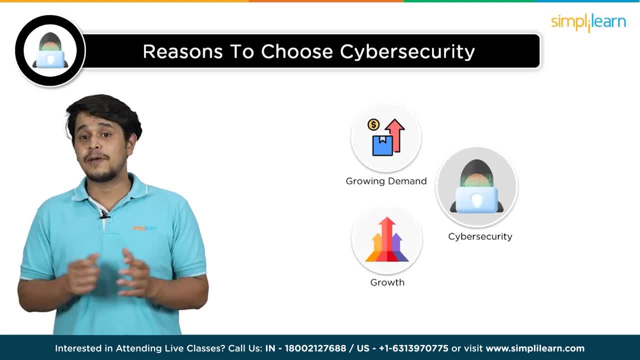 You will continually learn and grow while working in the field as a highly specialized skill. Market Variety: A career in cybersecurity enables you to leverage your passion for diverse industries. Despite the need for rigorous training, the skills gained can be applied across various sectors, including consumer-facing industries like retail. 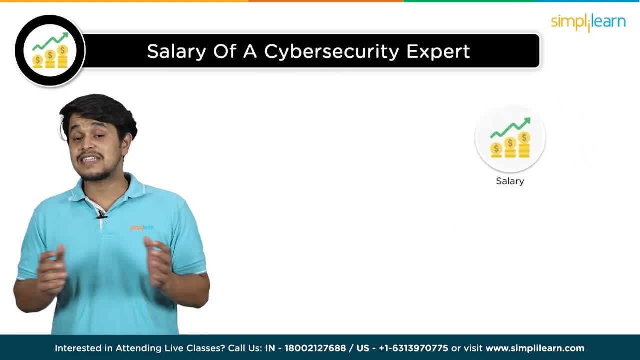 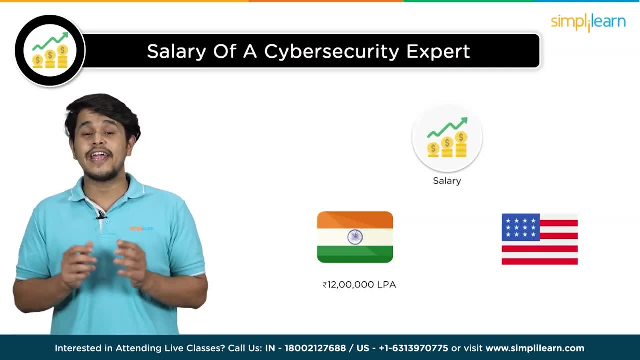 High Paying Salary. According to Glassdoor, the average salary of a cybersecurity expert in India goes around ₹12 lakh per annum, and the same in the United States. The average salary of a cybersecurity expert goes around $87,000 annually, with additional. 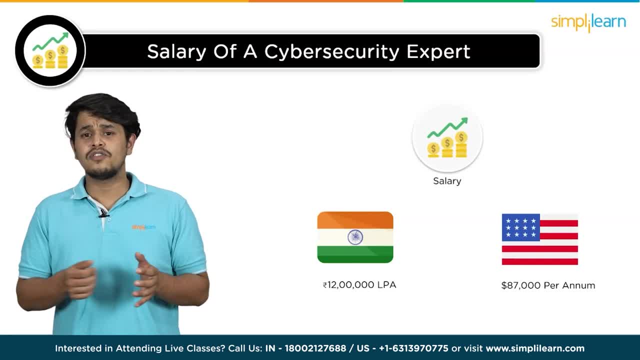 cash benefits. These are some of the main reasons why you should consider cybersecurity as your future. These salary numbers do not define your salary in any of these fields. Both fields are high-paying and it depends on your skills how much you'll earn in. 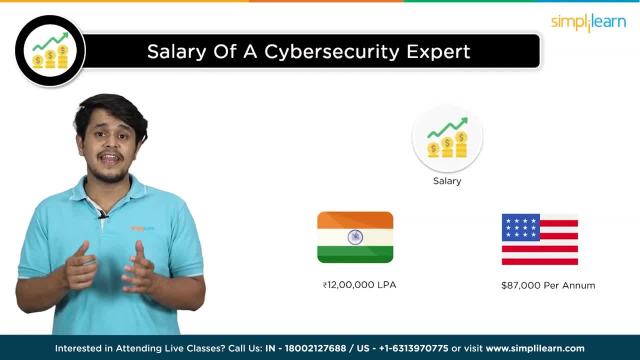 an year, How SimplyLearn can help you in mastering these fields. Furthermore, the last aspect is how SimplyLearn can help you in mastering these fields. SimplyLearn offers a wide range of certification courses for various technologies. For data science, it offers a wide range of courses. 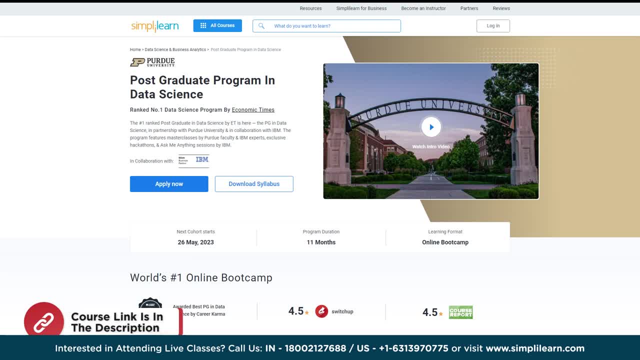 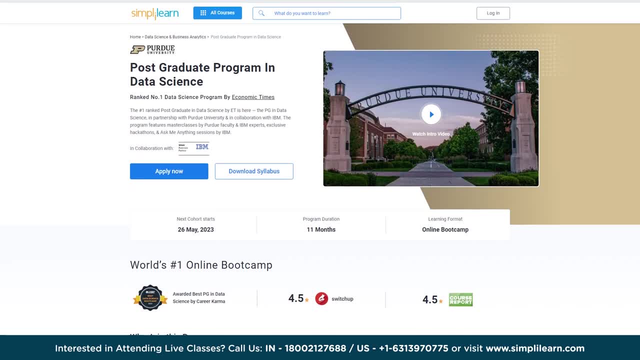 For software parts. it offers a wide range of services. For software parts. it offers a wide range of services. Practical Machine Learning. This is Microrical Data Science, the postgraduate programme in data science in partnership with Purdue University and in collaboration with IBM. 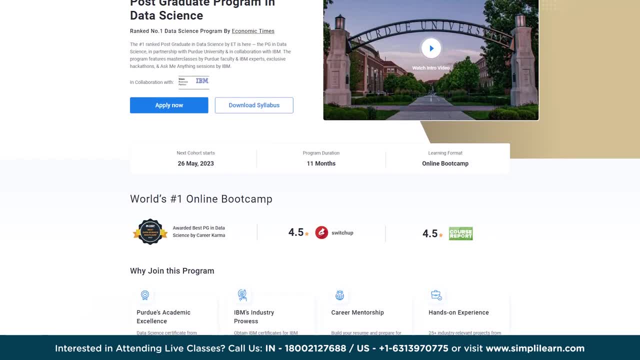 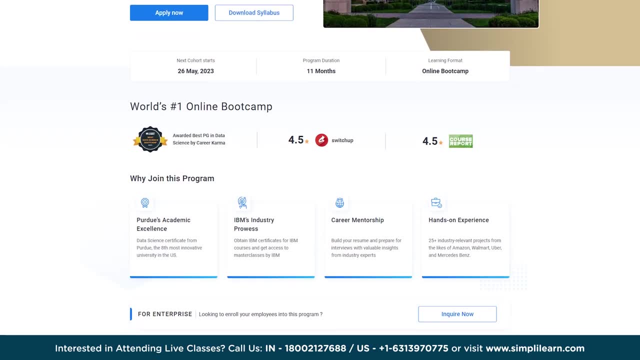 Features: masterclasses by Purdue faculty and IBM experts, exclusive hackathons and Ask Me Anything sessions by IBM. This in-depth postgraduate programme in Data Science is designed for working professionals. It covers job-critical topics like R, Python, programming, machine learning technique, NLP. 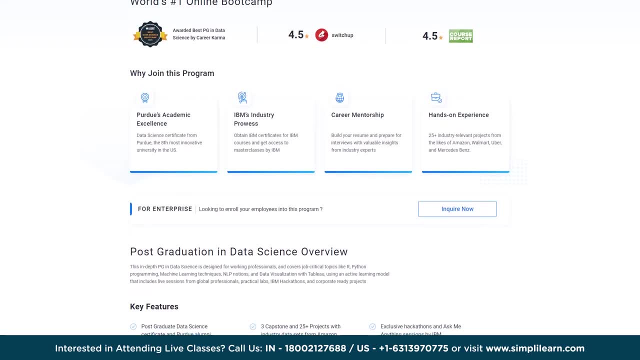 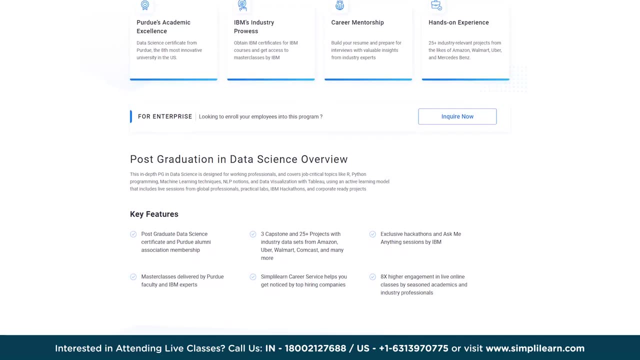 notions and data visualization with Tavaum. It uses an active learning model that includes live sessions, wirdge-aufgaben und weiter pizzeln이라고, live sessions from global professionals, practical labs, IBM hackathons and corporate-ready projects. 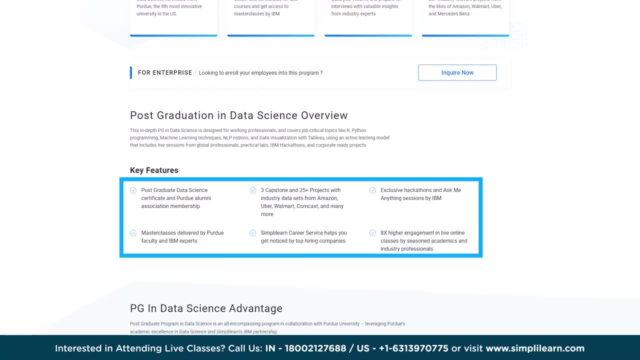 So what else can you expect from this program? Postgraduate Data Science Certificate and Purdue Alumni Association Membership. Three CAPS 10 and 25 plus projects within industry, datasets from Amazon, Uber, Walmart, Comcast and many more. Masterclasses delivered by Purdue U faculty and IBM experts. 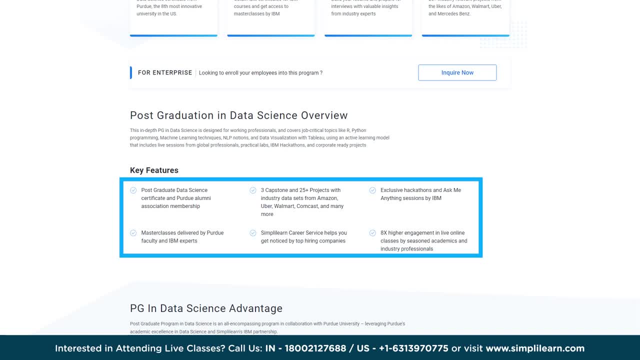 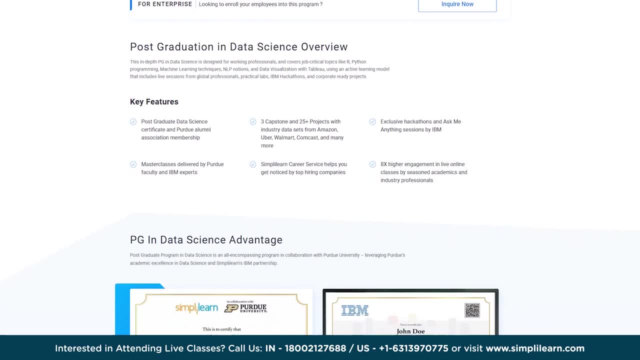 Exclusive hackathons and Ask Me Anything. sessions by IBM Simply Learns Job Assist. help you get noticed by top hiring companies. This postgraduate program in Data Science have a comprehensive course curriculum from Purdue University with a specialization in the following: Natural Language Processing. 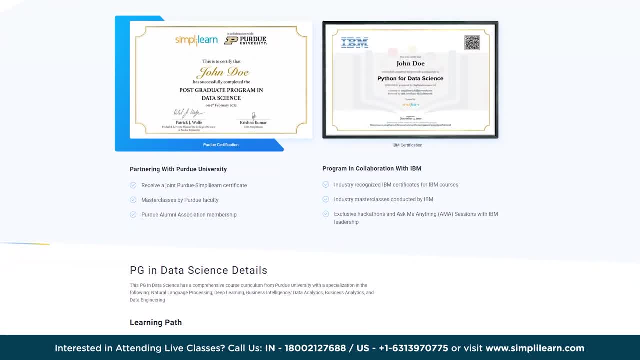 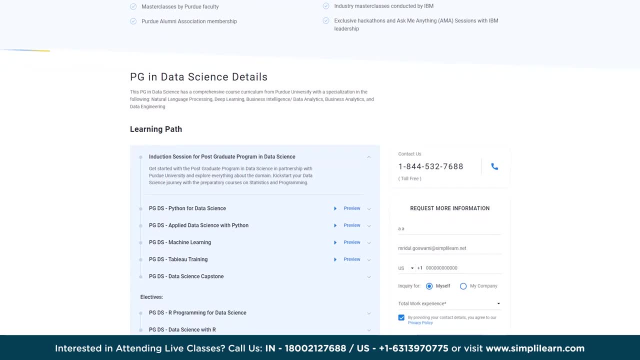 Deep Learning, Business Intelligence, Data Analytics, Business Analytics and Data Engineering. In short, this program offers a structured and guided learning experience that can help you build a strong foundation in Data Science and advance your career prospects in a rapidly growing field. So don't forget to check it out. 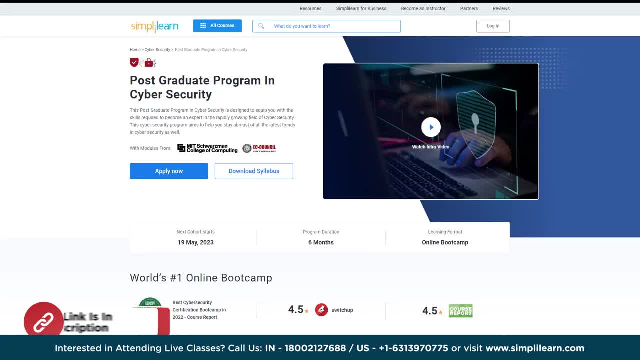 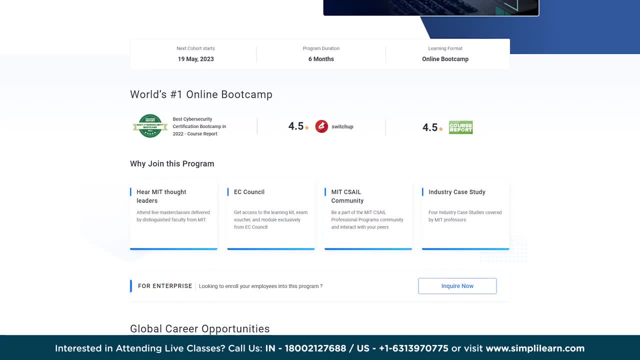 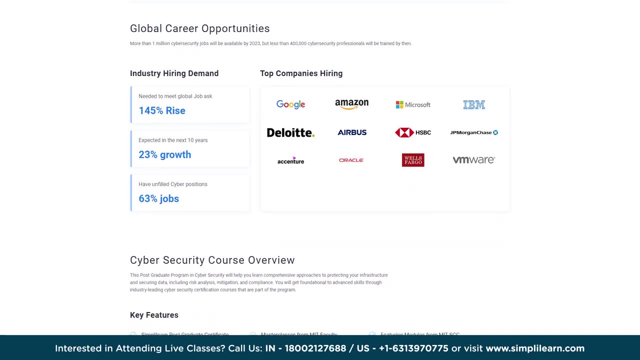 Check the link in the description box below. For Cybersecurity we have the Postgraduate Program in Cybersecurity. This program in Cybersecurity is designed to equip you with the skills required to become an expert in the rapidly growing field of Cybersecurity. This Cybersecurity program aims to help you stay abreast of all the latest trends in Cybersecurity. 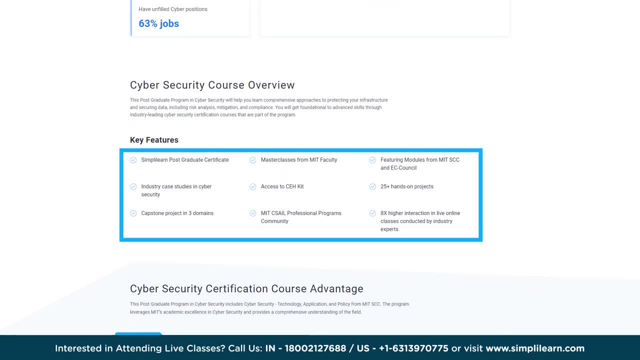 as well. Key features of this program: Simply Learn Postgraduate Certificate Masterclasses from MIT faculty, featuring modules from MIT, SCC and ECE. Access to Certified Ethical Hacker Kit. 25-plus hands-on projects and many more. 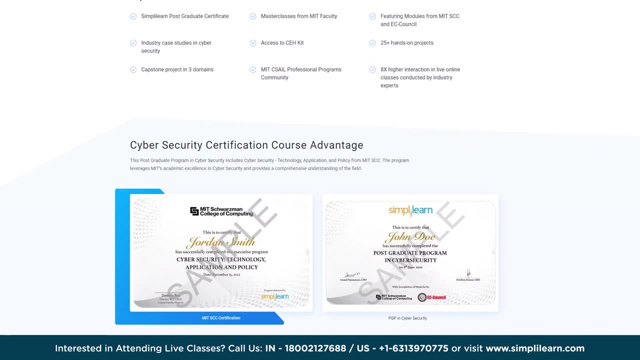 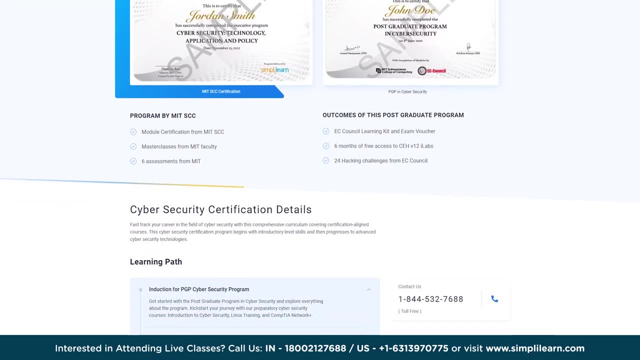 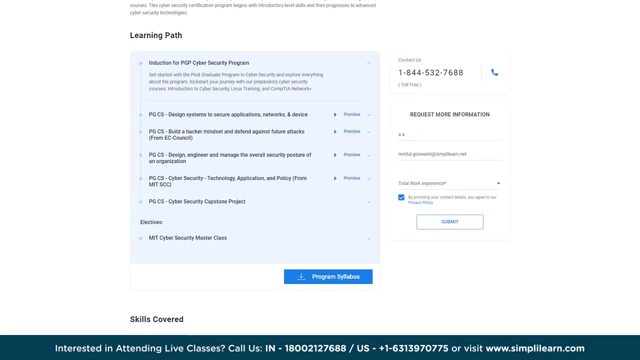 This Cybersecurity certification program begins with introductory-level skills and then progresses to advanced cybersecurity technology. Cybersecurity is one of the top concerns of businesses today, in any industry, From securing data to anticipating cyber attacks and placing enterprise-wide safeguards to prevent them. employers worldwide are increasingly looking for qualified cybersecurity professionals. 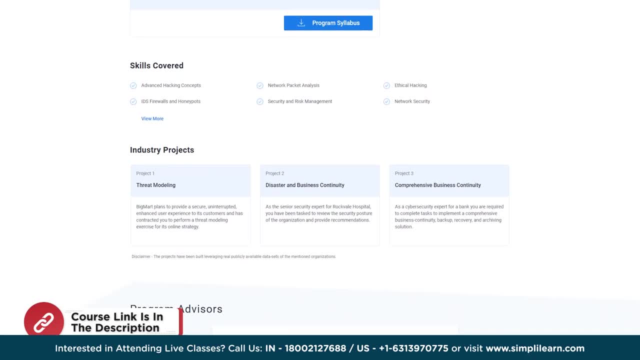 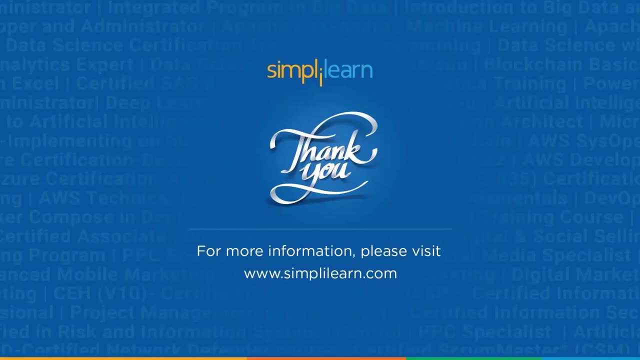 to join them, And I hope you now have a clear vision of which of these two fields you should choose for your career. Well, that's a wrap on Data Science or Cybersecurity- Which one you should choose? We hope you found this video informative and helpful.